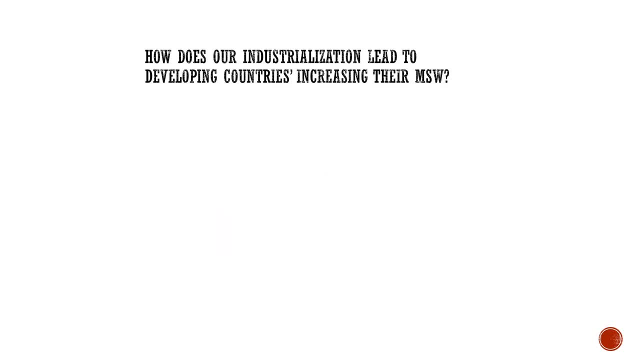 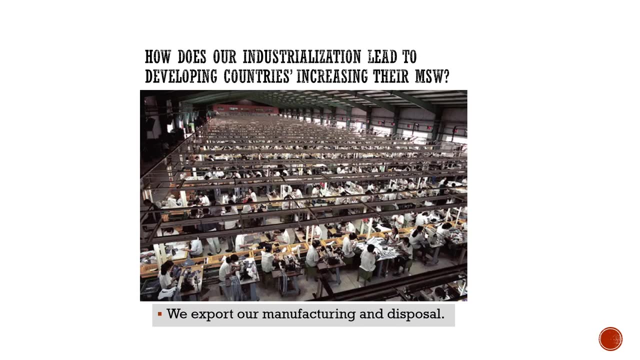 we're able to outsource those costs. So how does our industrialization lead to developing countries increasing their MSW? Well, we export our manufacturing at our disposal. We actually manufacture for most of the items that we use in an industrialized society. the manufacturing is. 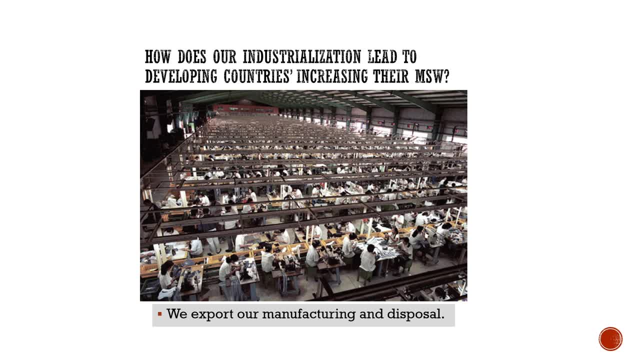 not done in the United States, for example. So we don't actually deal with the manufacturing and we also typically dispose in a different country as well. You know, your typical landfill obviously is going to deal with a lot of your waste. but all of those you know when we talked about. 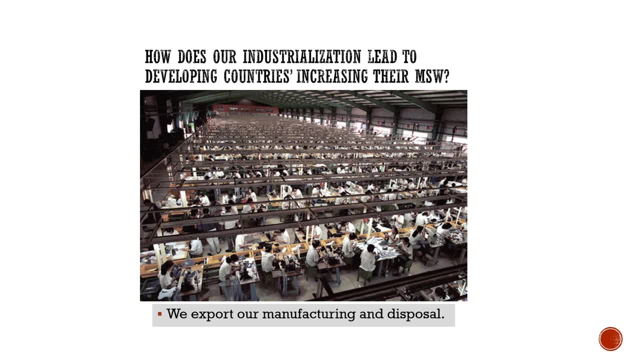 different types of waste and we looked at those things that had hazardous chemicals where they say, hey, don't bring this to the landfill, You've got to dispose of this in a different way. You can bring it to us, but we have to deal with it differently, So you can't just throw it in your 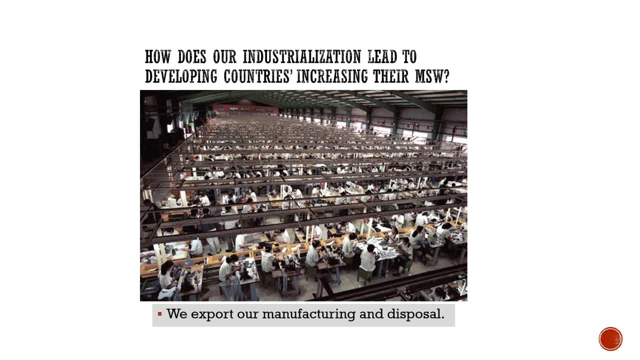 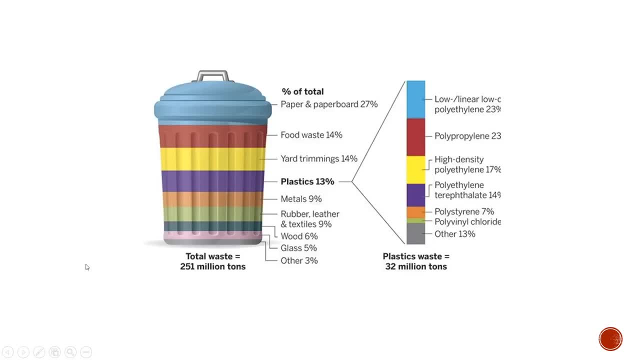 dumpster. What do we? what do they do with those chemicals? For the most part, they export it so that they can it can be dealt with somewhere else. So the total waste is 251 million tons. okay, That can be broken down into paper and paperboard, which is 27% of all of our waste. 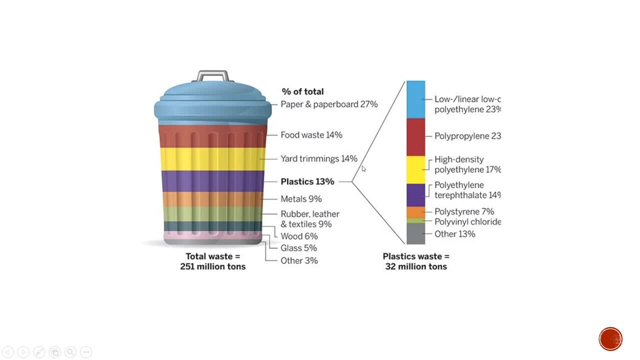 Food waste is 14%, Yard trimmings are 14%, Plastics are 13.. Metals are 9.. Rubber, leather and textiles clothing 9%. Wood is 6%, Glass is 5% And then other is 3.. So you can actually. 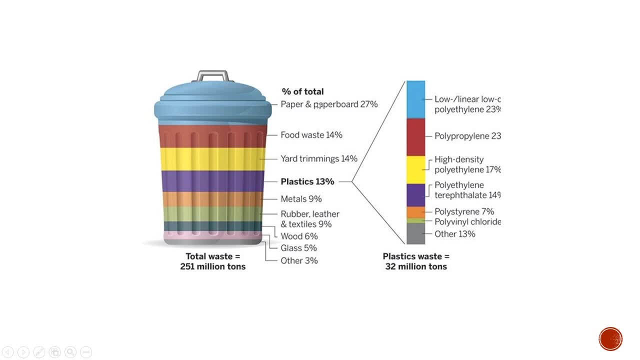 look at this waste and you can break this down and talk about. well, what is, you know, compostable, What is actually going to break down in a relatively shorter amount of time? Well, paper and paperboard, food waste and yard trimmings, which is nice because these are our top. 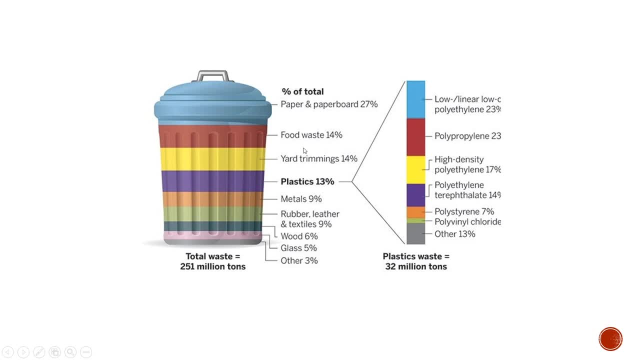 three sources of waste, So they will break down over time: Plastics, metals, rubber, leather and textiles. these three don't really break down in a very quick period of time. Wood does and glass does not, And then other, of course being other. Now, when we look at plastics, 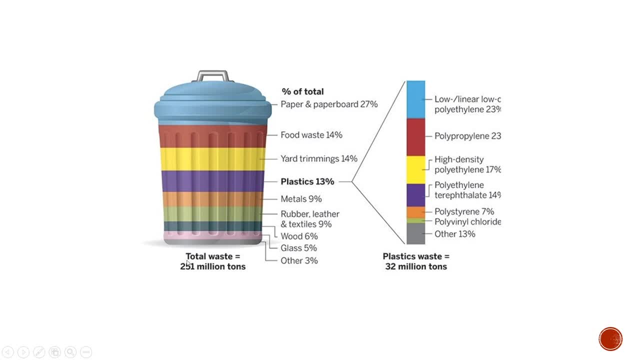 plastic waste is 32 million tons. You can do the math: 13% of 251 is 32.. I hope it is. this can actually be broken down into other sources, the sources of plastics, the different types of plastics we have: low linear, low carbon, polyethylene, polypropylene. 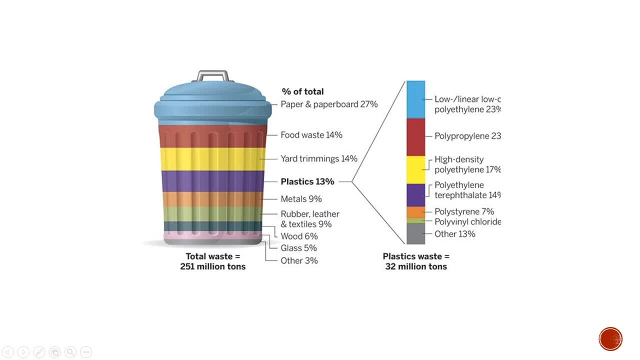 higher density: polyethylene, then polyethylene, terephthalate, terephthalate, oh good. polystyrene, polyvinyl chloride and then other sources of plastic. now, the reason we break plastics into their own different categories is because certain plastics can be recycled and 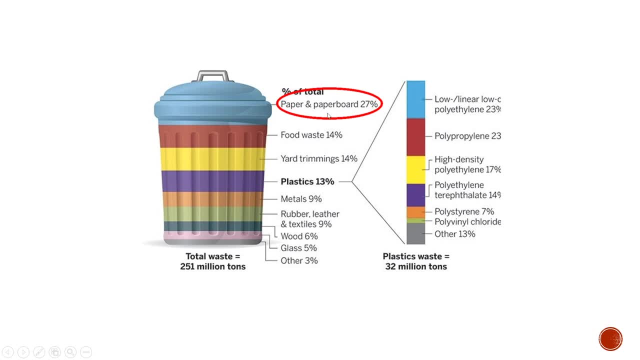 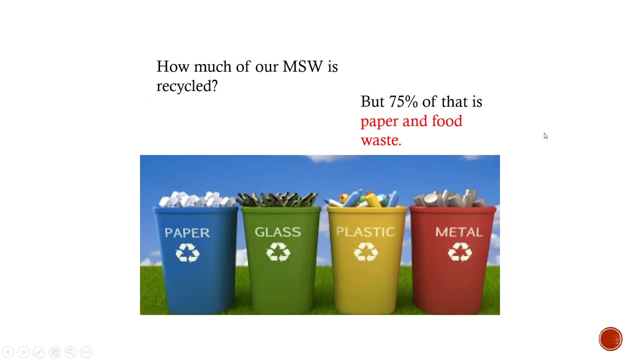 certain plastics can't, so we'll talk about that a little bit. but just note, paper and paperboard is the highest number of uh waste for us, food waste being number two. plastics is a huge one. so how much is recycled? okay, you, when we look at how much of our msw is recycled, 75 of that is food and paper waste. okay, so paper. 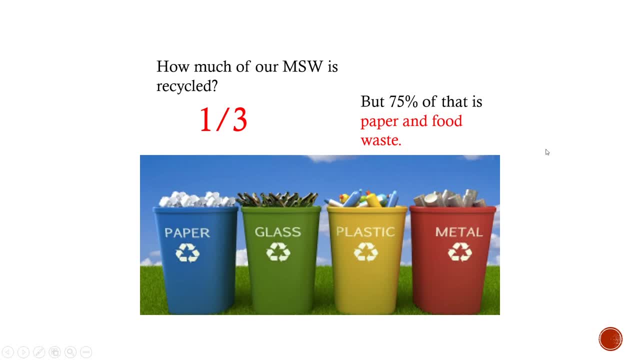 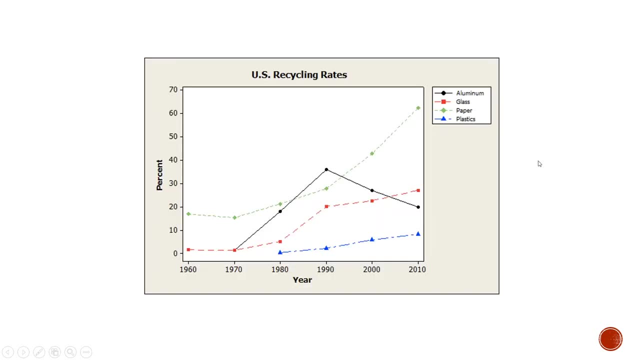 glass, plastic and metal. a third of our waste is recycled, keeping in mind that 75 is paper and food waste. now recycling rates in the united states since 1960: you know we look at the 60s and the 70s as being kind of our environmental. you know the green revolution here we actually saw a huge 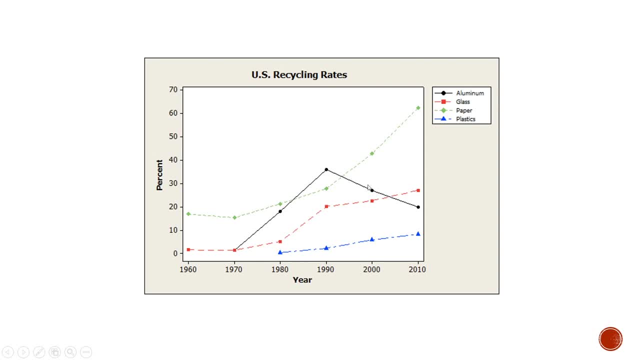 rise in recycling rates in the united states since 1960. you know we look at the 60s and the 70s as being Dick Gray's 죠, so we've- I'm going to talk about another run-up and that isdonan이드 rather callednous asmr. 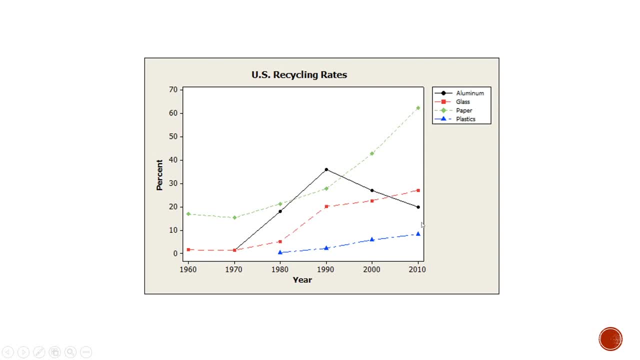 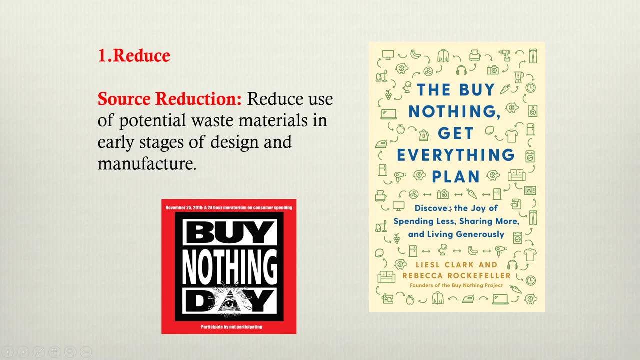 you know, we're looking at like 63% in 2010 of our paper was being recycled, whereas about, you know, 8% of plastic was being recycled. So we'll talk about some of the R's right. The first R is to reduce. This is the best thing we can do as far as dealing with 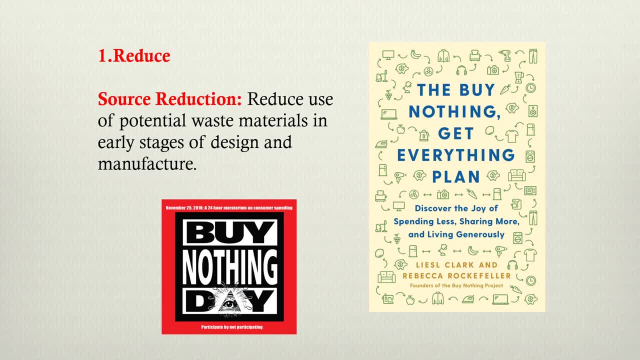 municipal solid waste is to reduce. If we use less of our source, we reduce the use of potential waste in the early stages of our design and manufacturing. So when we're designing things, when we're manufacturing things, we should always think about how can we use less of the sources to? 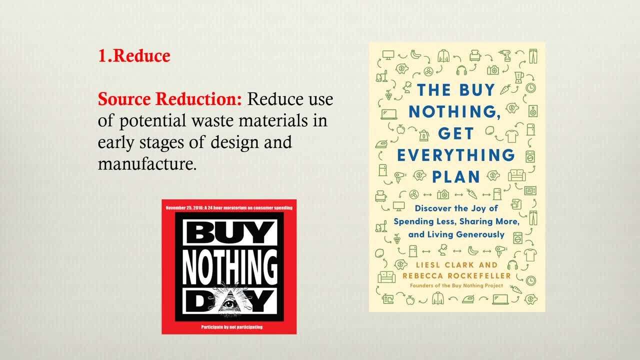 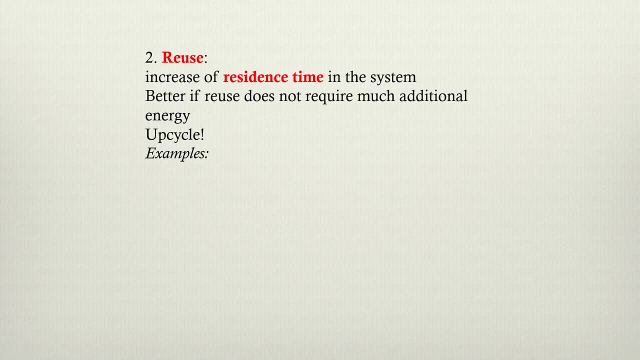 make these products. There's a great book called the Buy Nothing, Get Everything Plan, which is discover the joy of spending less, sharing more and living generously, but using less things. buying less and using everything. Then the second R is reuse right. By reusing items we can increase. 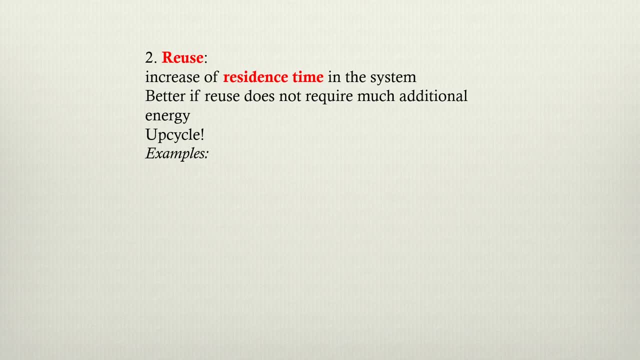 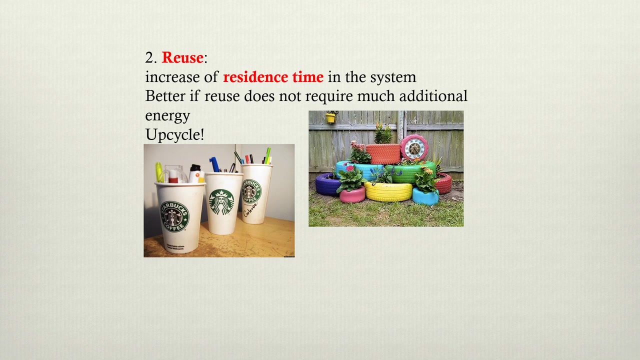 the residence time in the system. It's better if it doesn't require a lot of additional energy, which would be considering upcycling. So here's some examples. You know, use your old cups as holders for different items. You can use your tires to plant your plants. You know, those can be your planters. And then 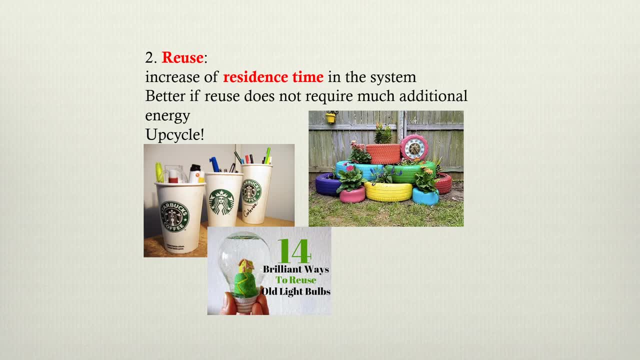 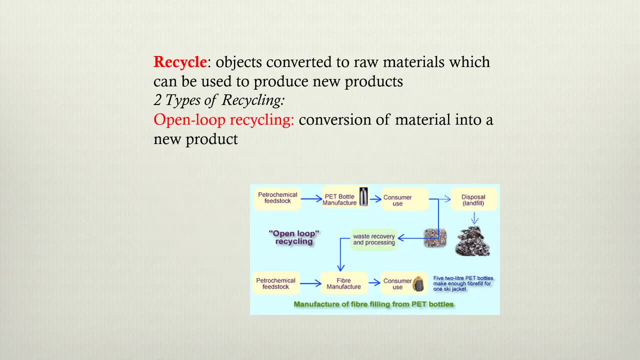 of course, there's things you can do to reuse your old light bulbs. You can use your old milk cartons as decorations. So there's a lot of things we can do in reusing. The idea of reusing is that you're not doing a lot of energy. 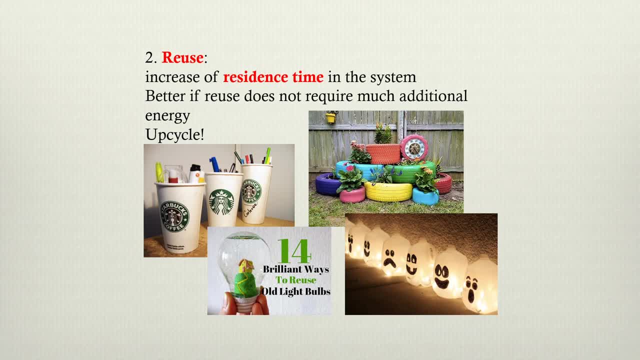 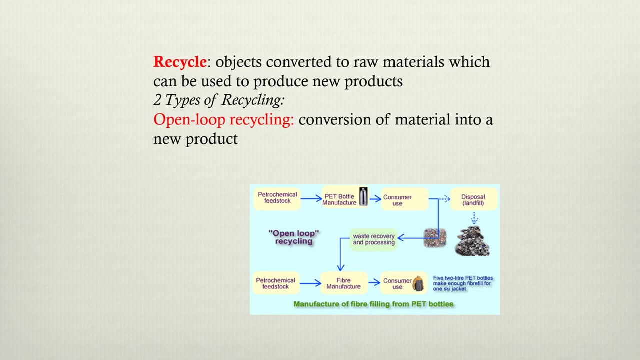 to reuse it. You're just upcycling it. You're using it for another purpose. Recycling is where we convert the raw materials back into the raw materials, where they can be used to then produce newer products. There's open loop recycling, which is where you convert materials into a new product. 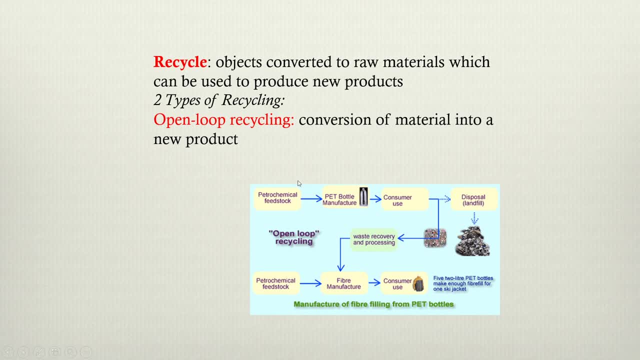 So here's an example of open loop cycling. So you have the petrochemical feedstock that create PET bottles, where they're manufactured. They're used by consumers. Now, some of them, of course, are used by consumers. Some of them are used by consumers. 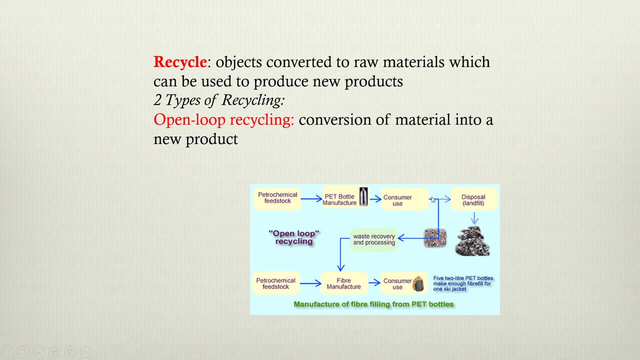 Of course are disposed in the landfill, But if they are recycled they can be recovered and processed and manufactured into fibers using more petrochemical feedstock to have another use from consumers. So two, or sorry five- two liter PET bottles make enough fiber fill for one ski. 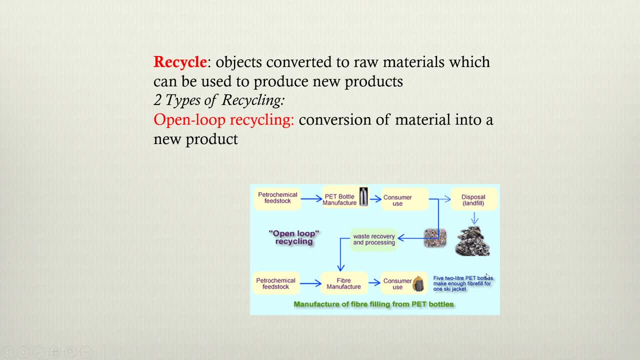 jacket, So you actually might see that if you're buying clothing, it might actually say on it: hey, this is used sustainably. We've we've reused Plastic to make this item And this is that process where you actually can manufacture fibers. 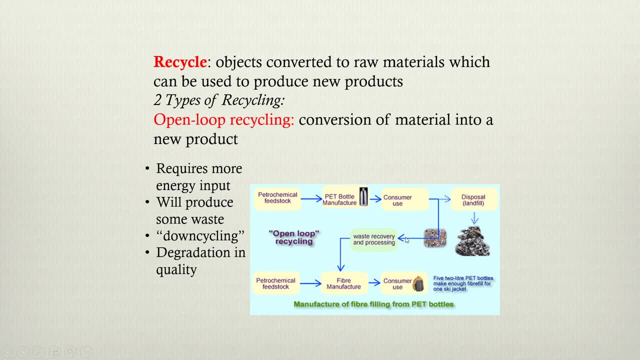 using those old bottles. Now, of course, this does require a lot of energy and it will still produce some waste If just reusing is considered. upcycling, recycling is downcycling because you're going down the process, You're not going to get as much of it And overall you're going to see. 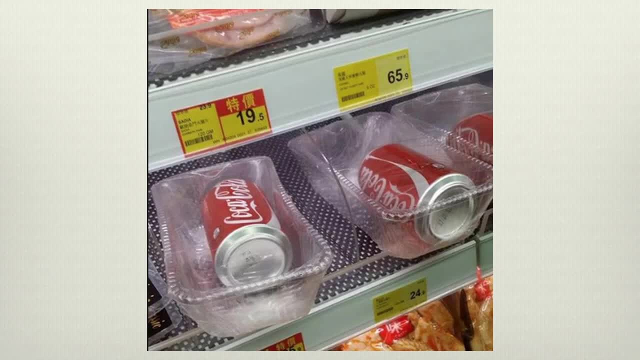 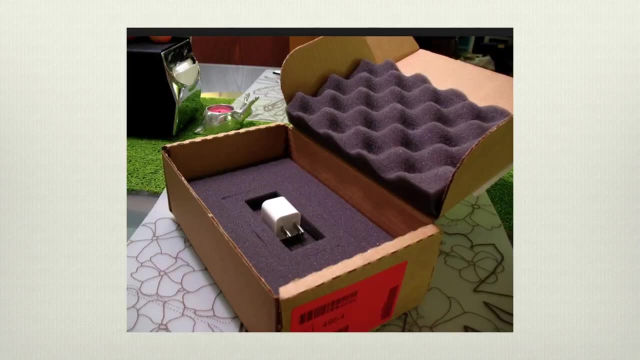 a degradation in the quality. Now here's some examples of maybe not so much degradation, but also great uses: Single use, plastic, of course, But these are just some of those examples of just ridiculous amounts of waste. Why Really Imagine you buy a new charger, a new wall charger, and it 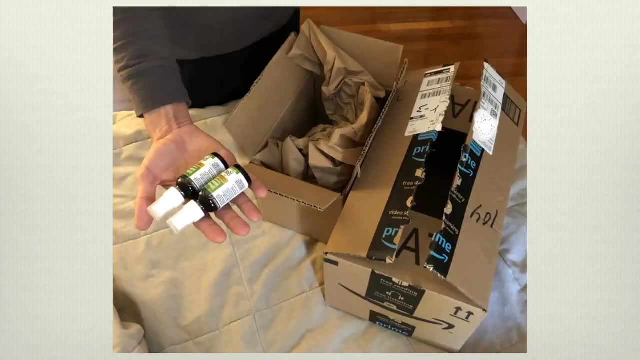 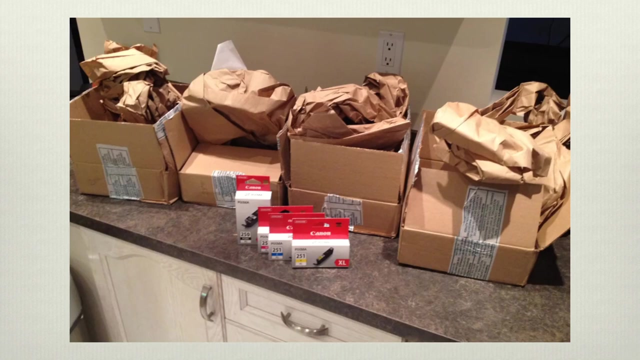 comes in that giant box for that A giant Amazon box with another big box inside of it with two small bottles. You know you've ordered something on Amazon and it's come like this and you just feel discouraged. So this is an example. Somebody bought some ink for their printer and each one of 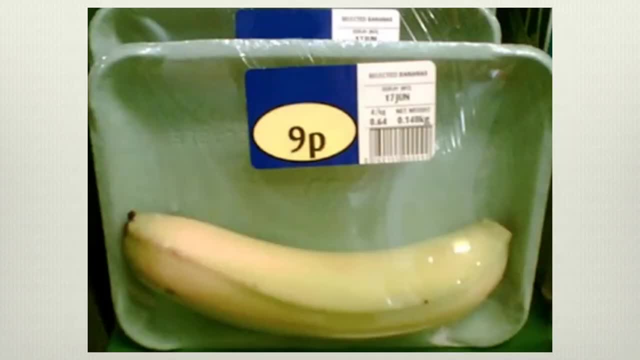 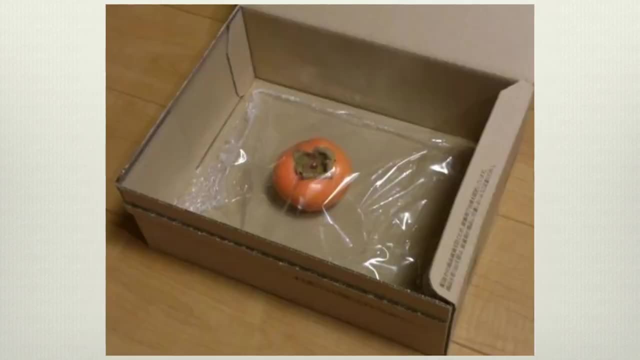 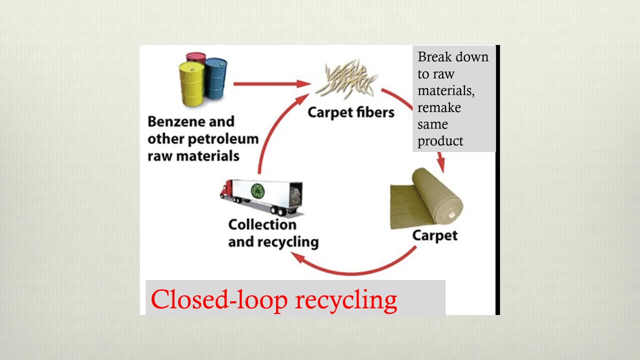 those little ink cartridges came in a big box. Why would you wrap a banana in plastic? It doesn't even make any sense. Oh, there you go, That'll keep it fresh. So closed loop cycling is a little bit different. where we can continue to use and reuse, Benzene and other petroleum are 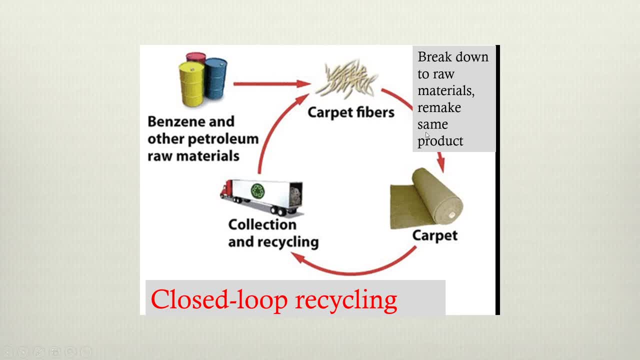 used to create carpet fibers, And those carpet fibers are then used in carpet And then you can recycle carpet. You can have it collected and recycled to make new carpet. So closed loop recycling is where you break down the raw materials and then remake the same product. 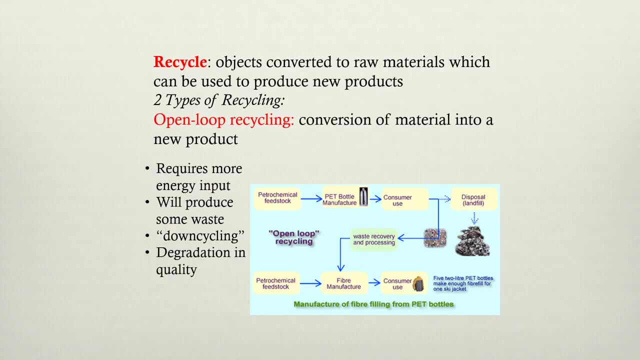 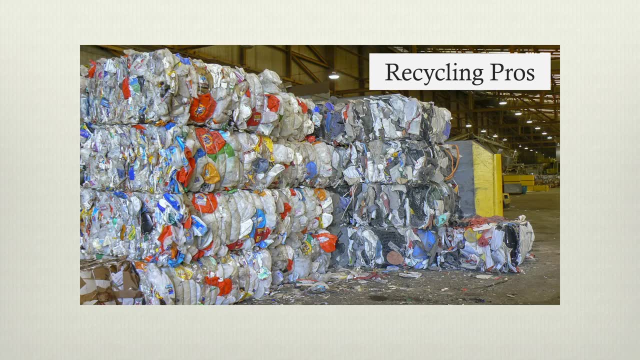 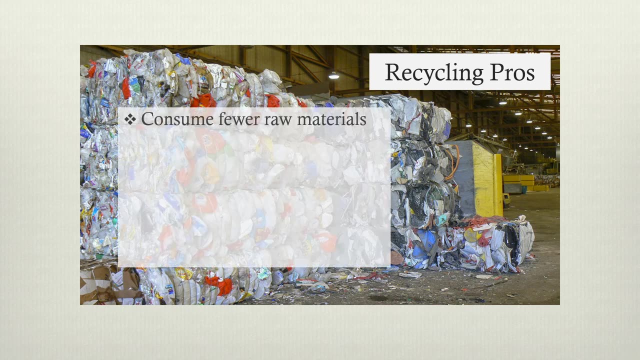 So remember open loop recycling. Open loop is where you convert it into a new product. Closed loop is where you use it to create the same product. So here's some recycling pros. We're going to look at some of the pros of recycling. Obviously, you're going to consume fewer raw. 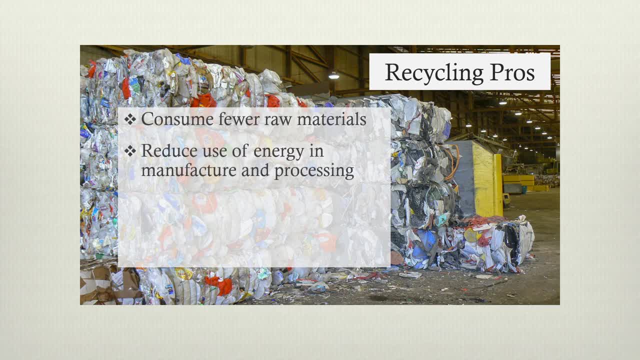 materials, You're going to reduce the amount of the use of energy in the manufacture and processing of those products. When you're creating products, you do use energy and you do have to process and manufacture. By recycling, there's less need of disposal, So you don't actually need as many landfills. 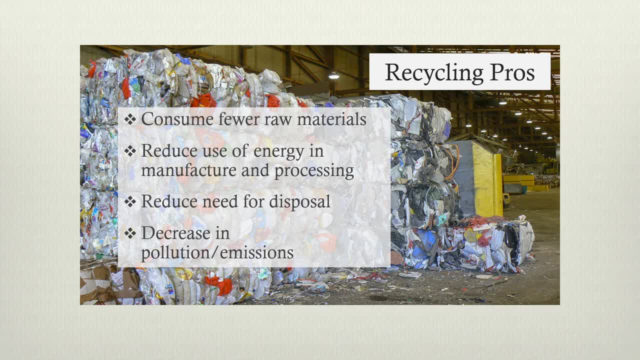 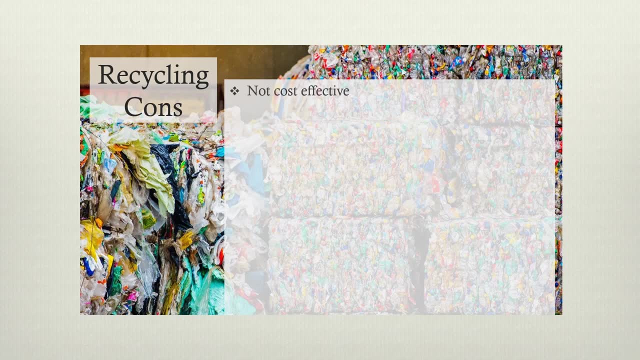 But overall it will reduce the amount of pollution and emissions. Of course there are always cons: It's not cost effective, And that is of course when we think about you know the real world we have to think about. can we make this cost effective? If it's not cheap, it's not going to. 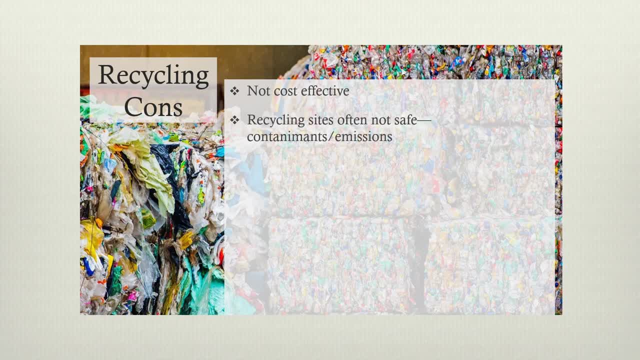 be something that's going to be done. They're usually going to have, you know, a lot of unsafe locations where they recycle because of contaminants and emissions. You have to remember that a lot of these products contain chemicals that can harm people, Usually the new products. 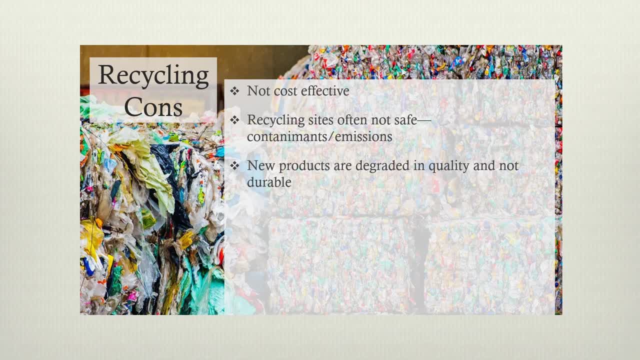 that are made are not as high in quality and they're not very durable. It's hard to implement this on a larger scale and in certain regions There's a lot of plastics out there that just aren't recyclable, And if they're not recyclable, you can't recycle them. 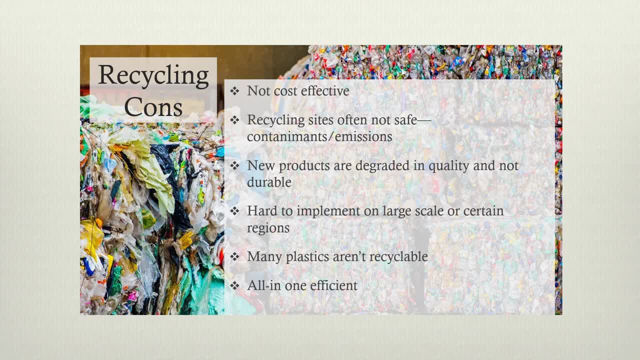 All in one efficient. I don't even know what that. why did I write that? Why is that there? And the biggest thing here is it's a false sense of security. We think of recycling and we feel good about it. right, Because recycling we're. hey, I'm doing my part. In reality, you have to. 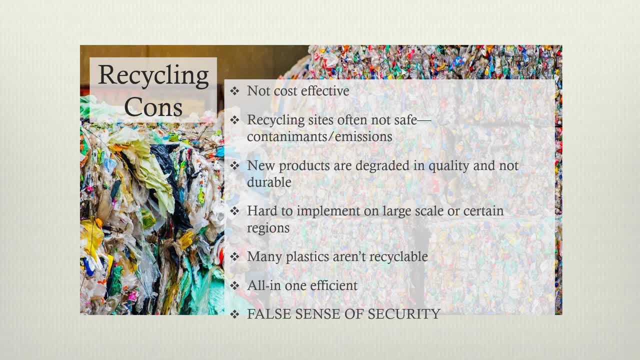 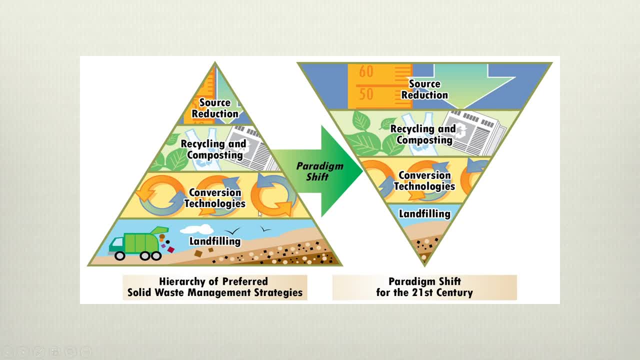 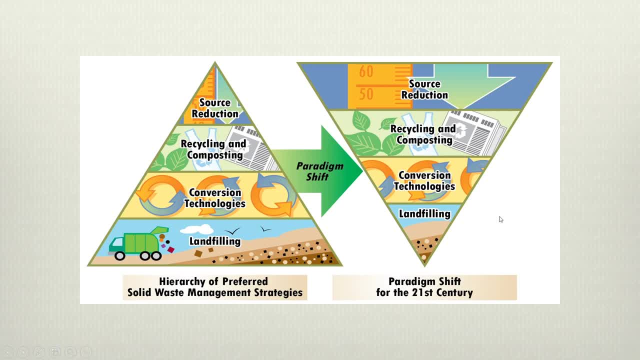 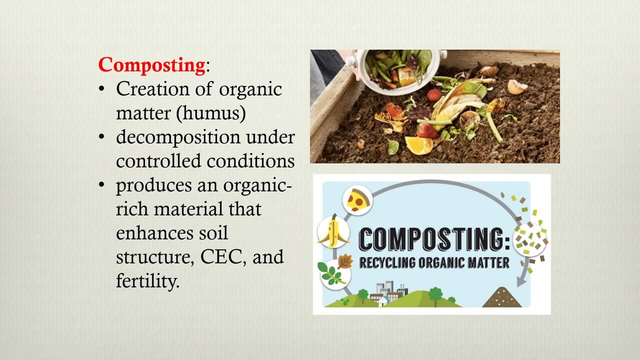 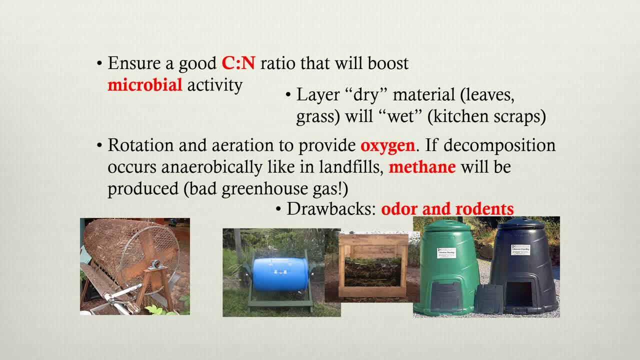 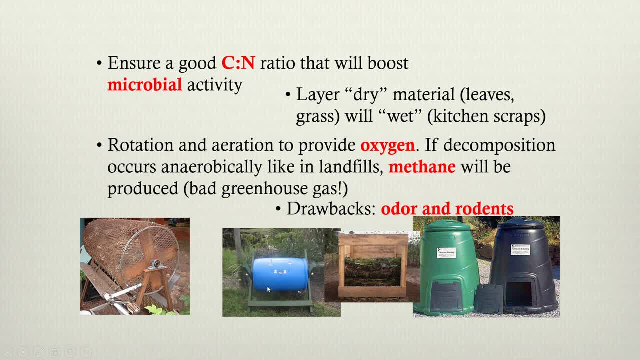 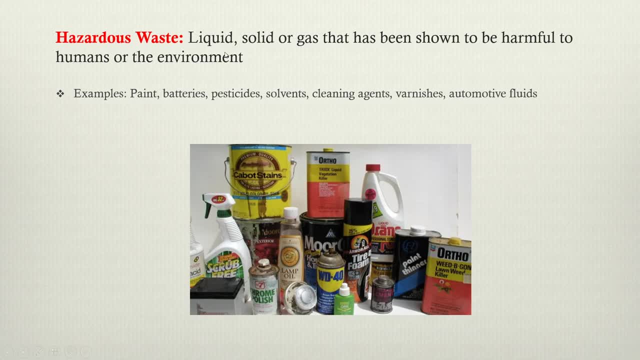 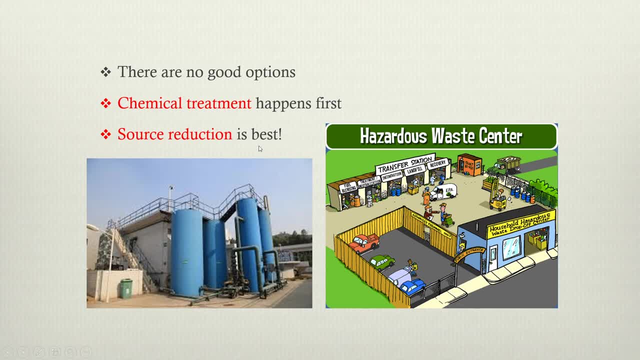 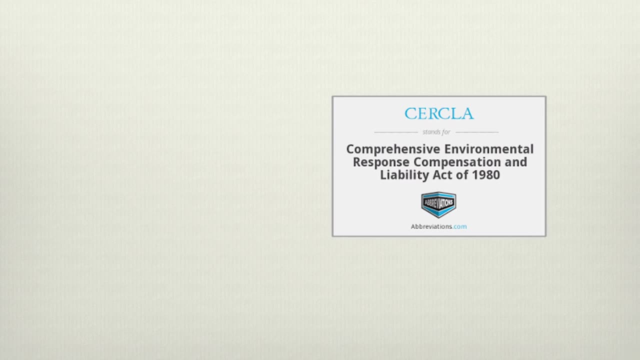 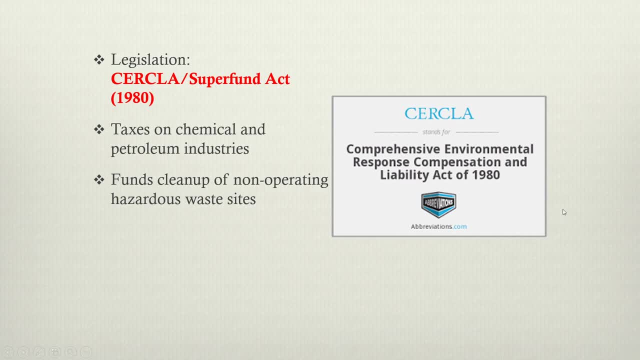 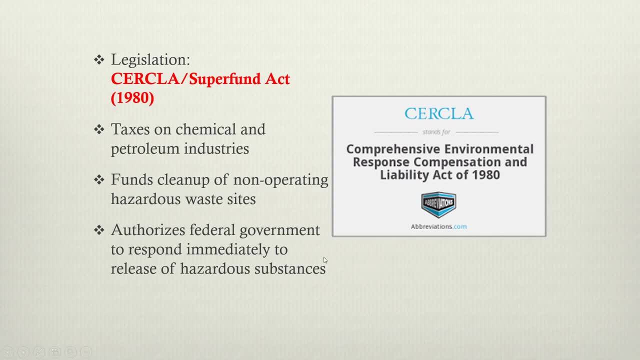 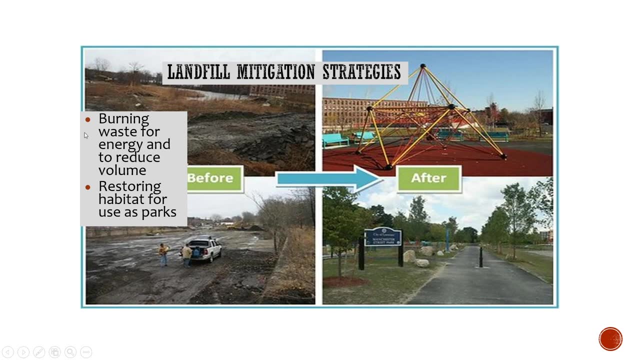